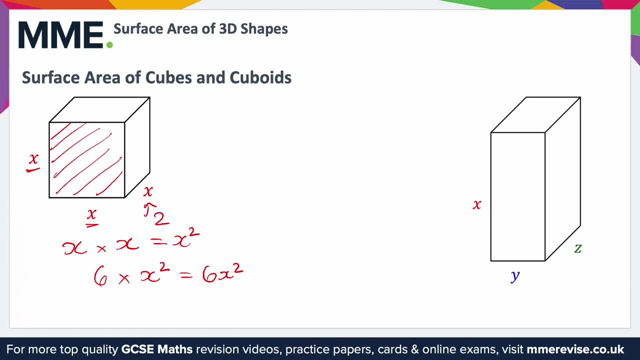 then the surface area is 6x squared. So I can just add an example into this. So for the surface area, I can just add an example into this. So, for example, if I make x 2, area of a cube with side length, 2 would be 6 times 2 squared. 2 squared is 4. so 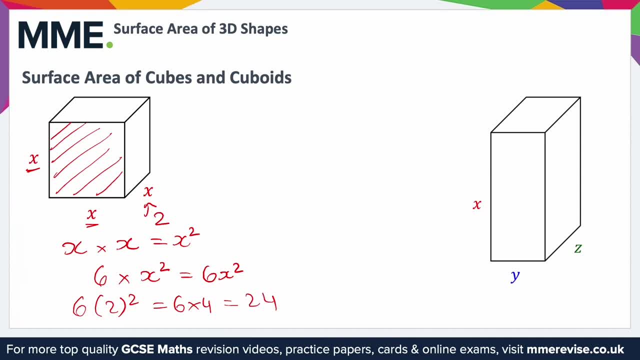 this reduces down to 6 times 4. 6 times 4 is 24, and then of course add whatever unit, so it could be centimeters squared, meters squared, etc. the surface area of a cuboid is a little bit more difficult just because you've got three pairs of. 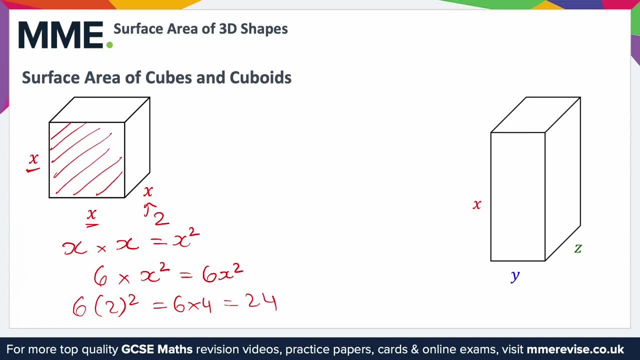 different size sides. the issue is here. you can see that this side is not the same as this side, which neither are the same as this side. okay, so what we need to do is work out the area of this side, the area of this side, and then the area. 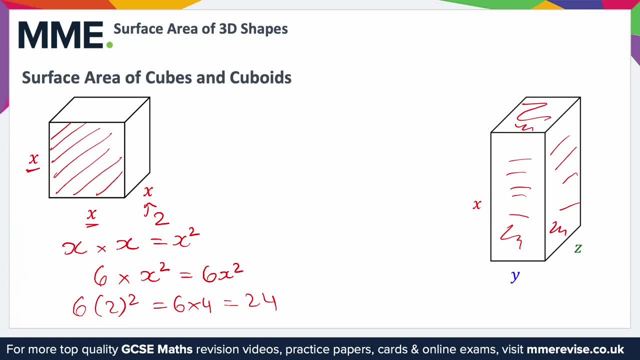 of this side and then, nicely, we know that there's two lots of each of those, because if we're talking about this side, then the side over here on the left would be the same. if we're talking about this front side, then the back that we can't see would be the same. if we're talking about the top and the bottom, 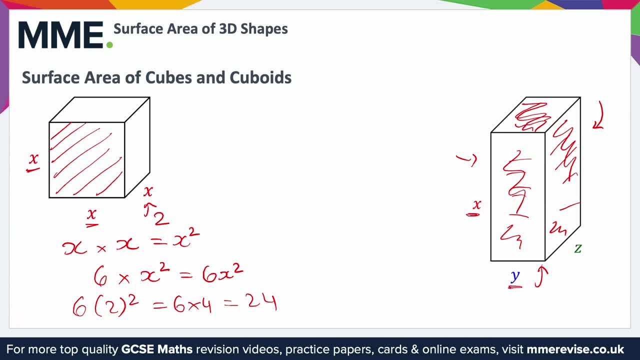 will be the same. So, looking at the front, it's X tall and Y is semi-tall and y wide, So the area of this side will be xy. So there's one side. Then, if we look at this side over here, it is z wide and x tall, So it's going to be xz. And then finally, the top, It's not. 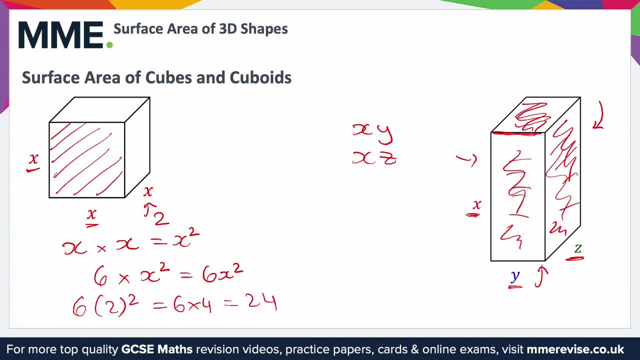 immediately obvious, but we know that this side will be the same as this, So we know that that's y, And the depth of the cuboid is the same as here. So we know that this is z, So it'll be yz. 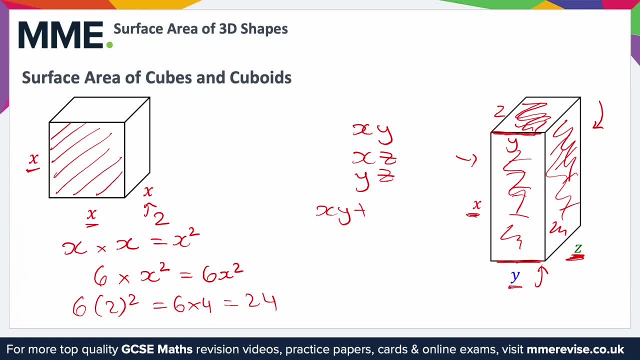 So, adding all of these up, you'll get xy plus xz plus yz. But remember there's two lots of each of these, because the top, of course, there's a bottom, which is exactly the same, The front there's a back, which is exactly the same, And the right hand side there is a left hand side. 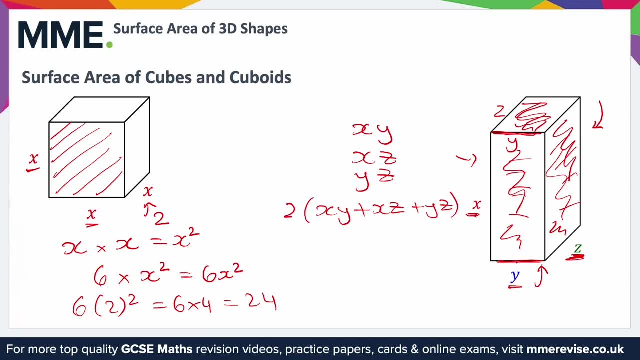 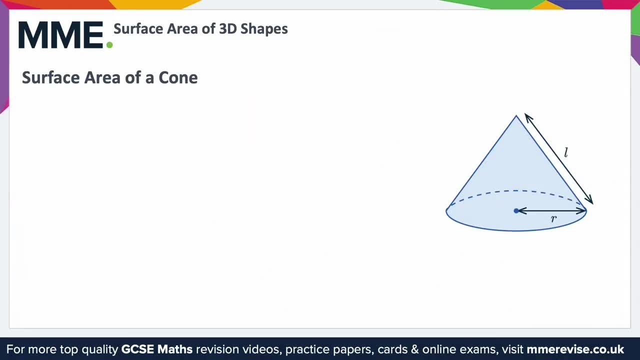 that's exactly the same. So just times this by two And then that will give you the surface area of the cuboid. The surface area of a cone is a little bit tricky, but you can split it into two parts. You could imagine it as the base here, which is just a circle, And we know the area of a circle is just. 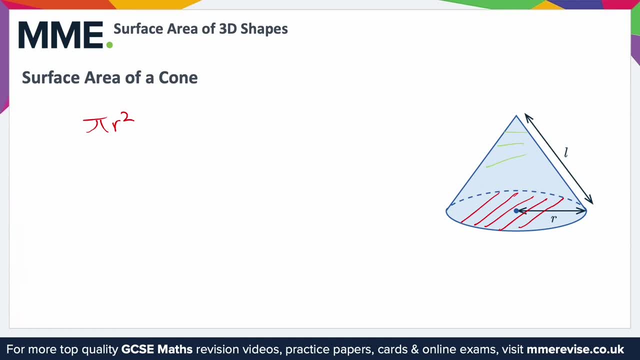 pi r squared, Then we could imagine this sort of curved bit that wraps around. This one's going to be really tricky to sort of derive what the answer is going to be. However, we can deduce that it ends up being pi r squared, So we know that the surface area of a cone is a little bit tricky. 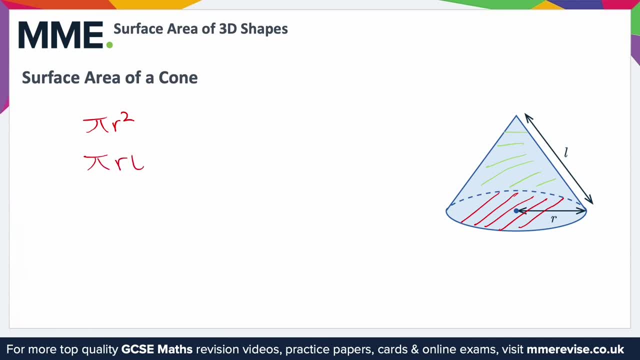 but you can split it into two parts. You could imagine it as the base here, which is just a circle, So r is the radius, remember, Pi is just the constant 3.14, and et cetera. It carries on. 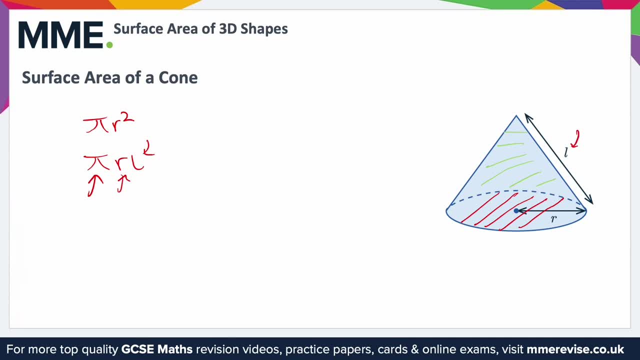 forever. And then l is this slant height here. So the total surface area you just add these two together: pi r squared plus pi r l Surface area of a cylinder. again can be a little bit tricky to spot what you need to do, But let's focus on the shapes that we can deduce So clearly. the two. 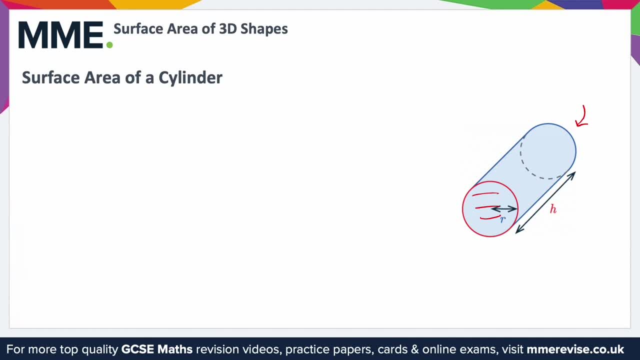 ends are circles. So we can deduce that the surface area of a cone is a little bit tricky. but we can deduce that the surface area of a cone is a little bit tricky, So clearly the two ends are circles. So it's going to involve pi? r squared somewhere. But how can we work out the middle bit? Well, the 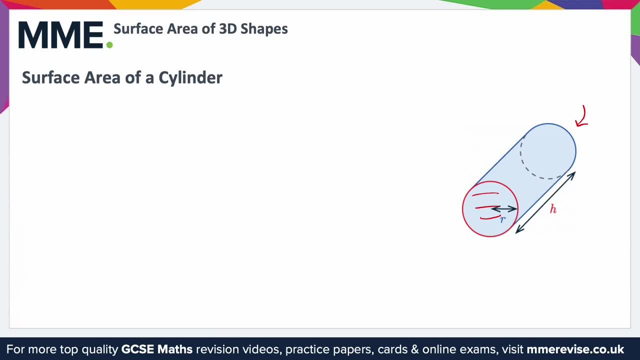 middle bit. if you think of origami, if you wanted to make a tube, you've effectively got a rectangle that you've rolled up to make a tube So we could split this shape up into its net, which is something a little bit like this: So you can see, there's two circles and then a rectangle in the 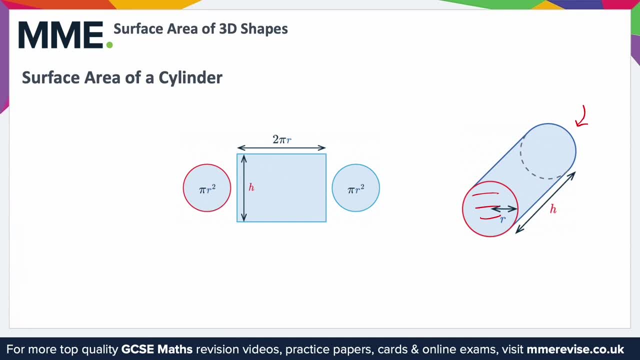 middle. So if we can work these out individually- the rectangle, the two circles- then we just need to add them all up. So the circles we should know are the ones that are going to be the most visible. So we know that those are pi r squared for each one and there's going to be two, lots of. 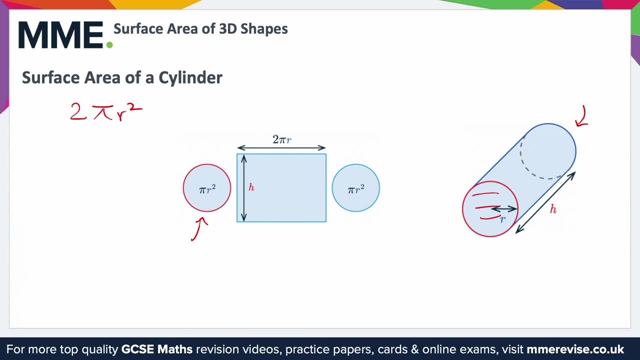 that. So it's going to be two pi r squared, Then the rectangle in the middle. it's not immediately obvious, Obviously. we know the length of it. That is just this here. But we don't know the width of it. So the width is just the distance around the circle, isn't it? Because it spans all the way. 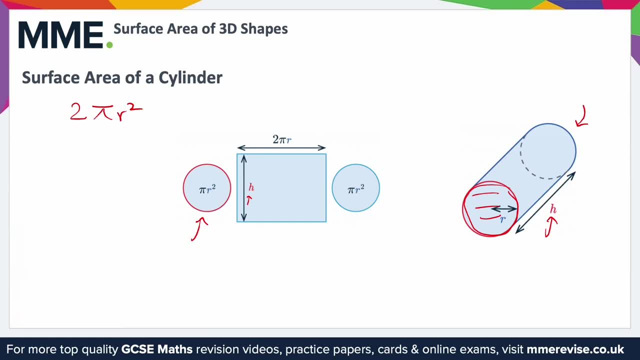 around, which is the circumference of the circle which, as we know, is two pi r. So, to work out, the area of this rectangle would just be two pi r h. So the total surface area of this cylinder would be two pi r squared plus two pi r h which, if you really